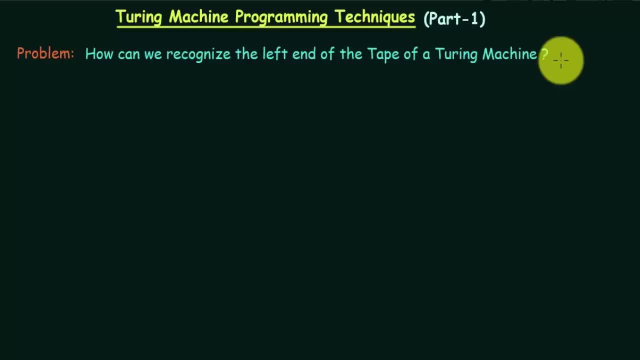 Or sometimes, when we reach the left end, we are required to move one step to the right, or something like that. But the question is, how can we know that we actually reached the left most end of the tape of a Turing machine? So we always say that we have reached the left end of the tape. 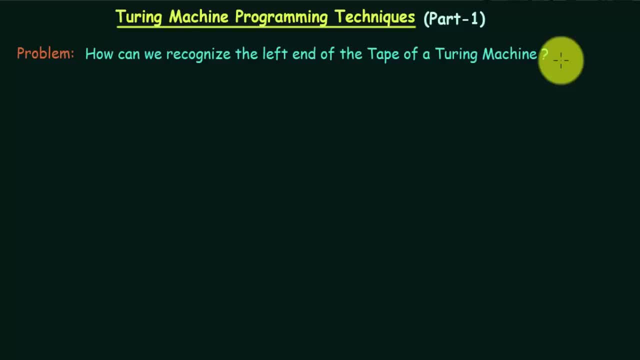 But how does the Turing machine know that this particular cell is the left most end of the tape? So there is no inbuilt technique, or there is no inbuilt method in the Turing machine that helps it to understand that it is at the left most end. 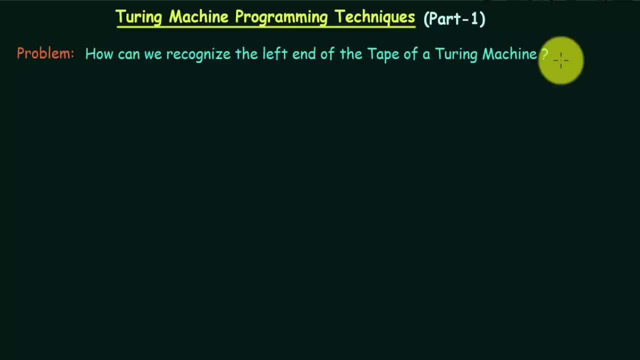 So what we want to do is we want to find a solution to this problem And we want to program our Turing machine in such a way that, if it is at the left most end, it will know that it is actually at the left most end. 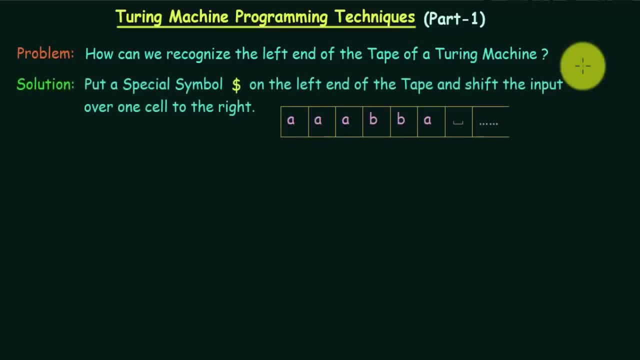 So let us see what is the solution that we can have for this problem. So here is the solution that we can have. The solution says that put a special symbol, like a dollar symbol, on the left end of the tape and shift the input over one cell to the right. 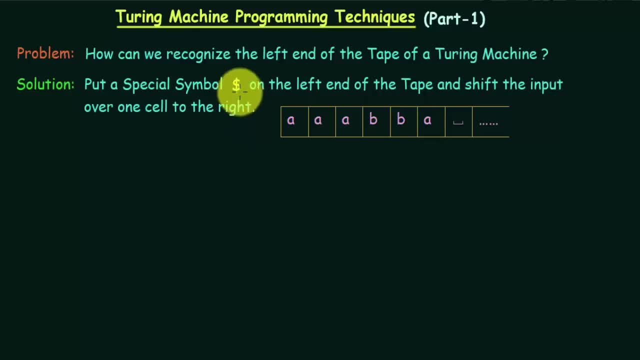 So this is the solution that we can have. What we can do is that on the left most end of the tape we will put this dollar symbol And then the rest of the symbols which are there. we will shift them one step to the right. 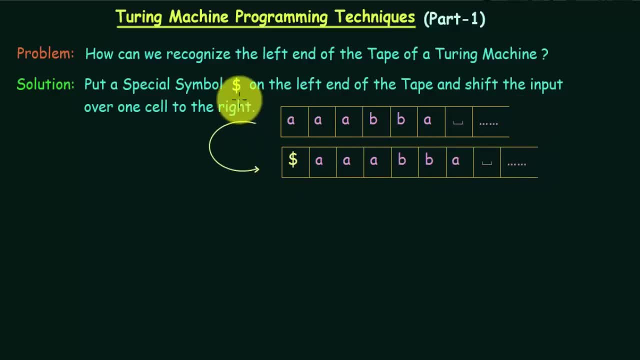 So it will look something like this: So here we put the dollar symbol on the left, most end, And then the rest of the symbols. we just move them one step to the right. So even in our push-down automata, when we had the stack, 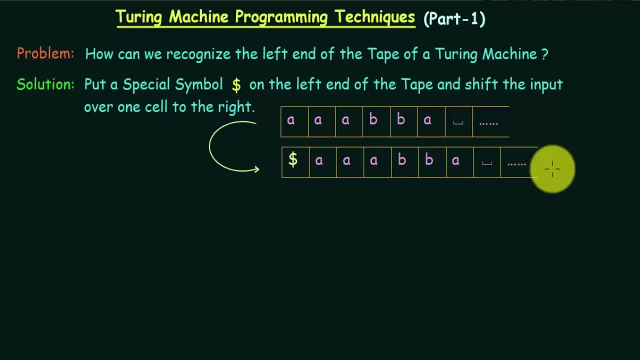 we used to put a symbol on the bottom most cell of the stack in order to denote that it is the bottom most element, or in order to denote that when you reach that element, you know that you have reached the bottom most element of the stack. 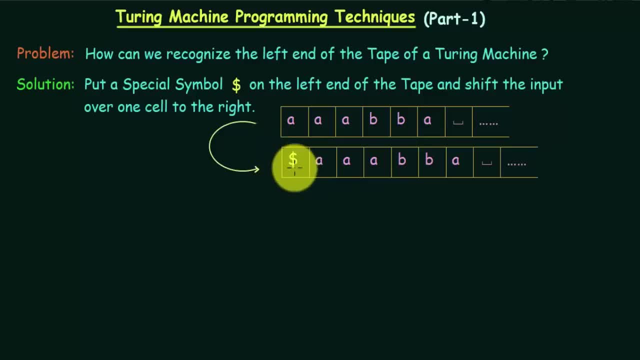 So, in the same way, if you put this dollar symbol on the left most end, then we can know that whenever you encounter this dollar symbol, you have reached the left most end of the Turing machine's tape. So this is one solution that we can have. 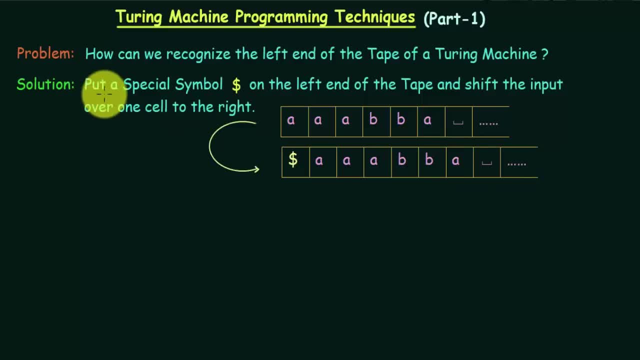 Now the question is: how can you design or how can you program your Turing machine in such a way that it will perform this task? So suppose let's say that we have a Turing machine which is going to perform a particular task, or which is there to decide a particular language? 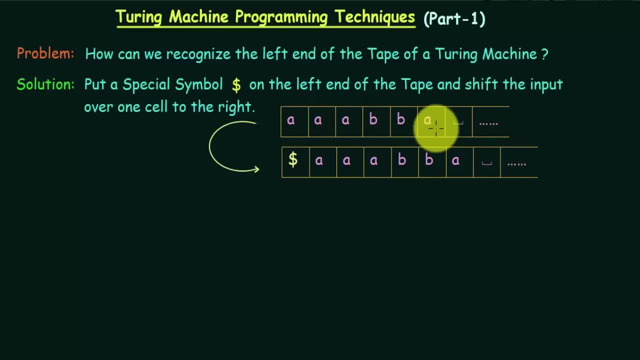 And then it has a tape like this with some symbols in it, And now we want to put this dollar symbol at the left most end and then move every other element one step to the right of the tape. So how can we have a Turing machine which will perform this particular task? 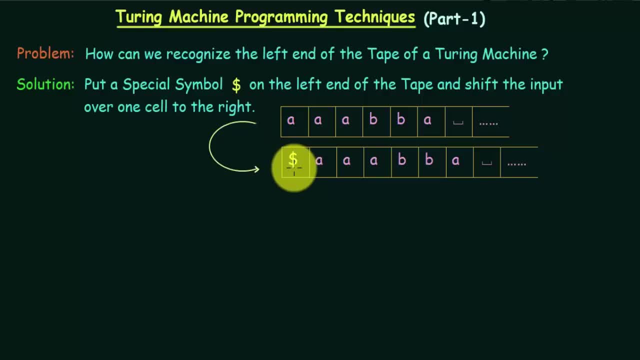 of putting the dollar symbol at the left most end and moving the rest of the symbols one step to the right. So let's see how we can design or program our Turing machine in order to do this particular task. So here I have designed the Turing machine which will perform this particular task. 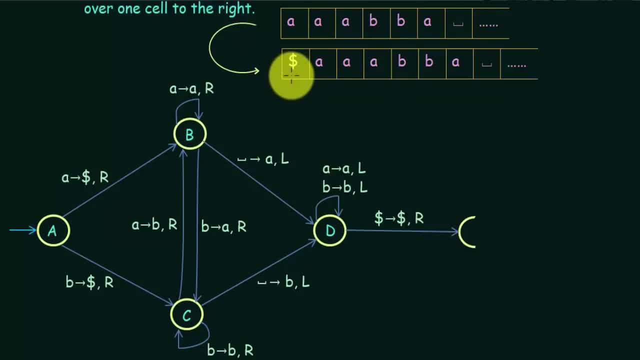 of putting the dollar symbol at the left most end and moving the rest of the symbols one step to the right. Now let's see how this Turing machine works. So here we have four states: A, B, C and D, And this is the state that follows. 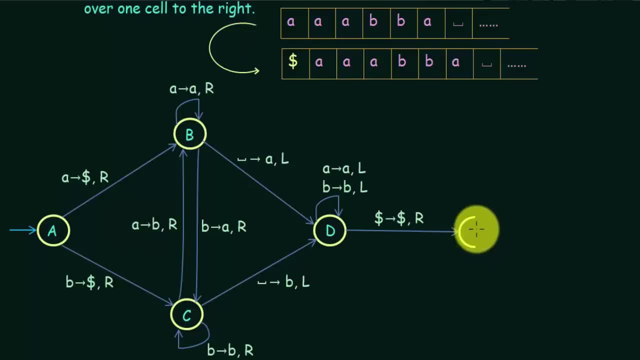 So what is this? I will explain it to you as we proceed. So first of all, let's see: Here we have the starting state A And in the starting state A we see that if you see the input symbol A on the tape, 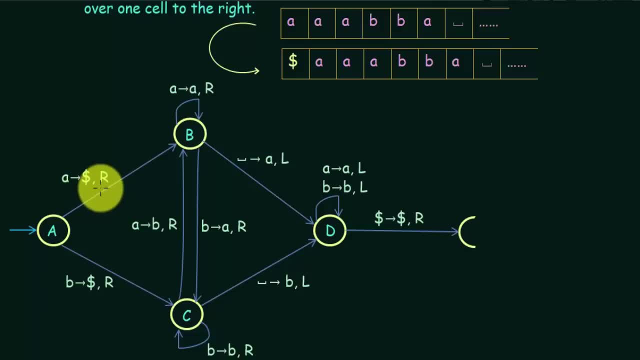 then you replace that A with the dollar symbol and you move one step to the right. So just like this Here: if you see an A, you replace this A with the dollar symbol over here and you move one step to the right. Alright. 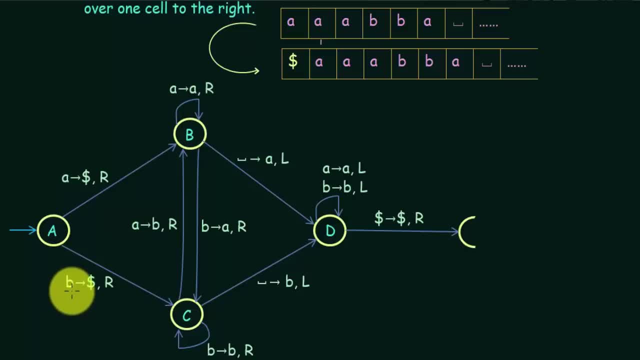 And we see that if you get a B or small b, if you see a small b in the tape, then also you replace that B with the dollar symbol and you move one step to the right. Now, why we are doing this is because 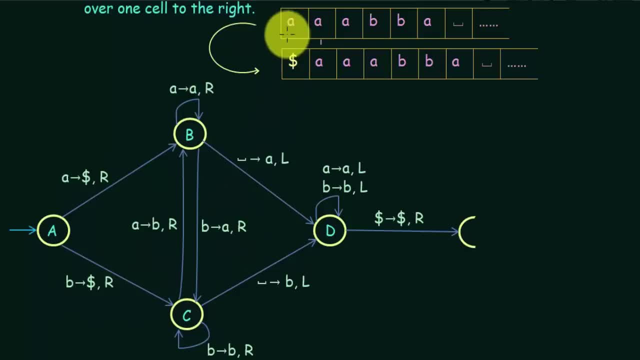 we are not designing this Turing machine in order to work only for this particular input symbol. So here we have this input symbol: A, A, A, B, B, A. So we are not designing this only for this, but we are designing this Turing machine. 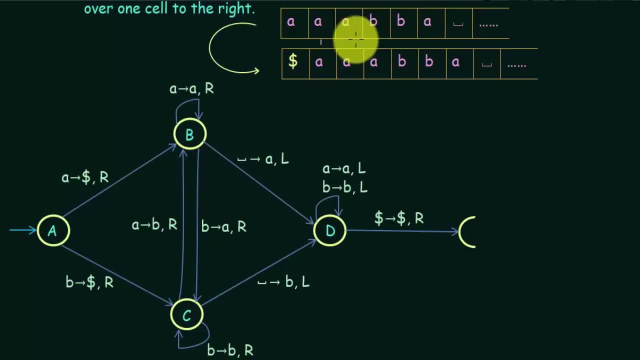 which will work for any kind of input symbols that we have over the alphabets A- B. So even if you get B in the beginning of the tape, then you replace that B with the dollar symbol and you move one step to the right. 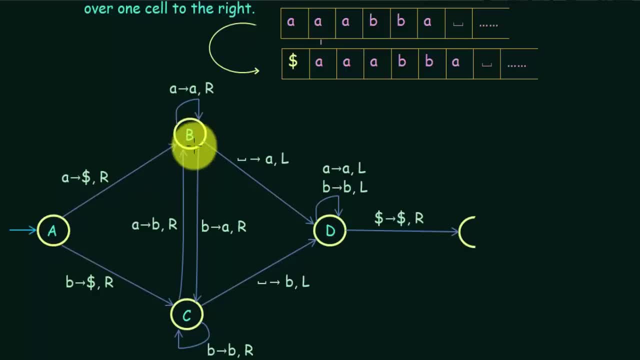 Alright, Now let's come here. Now we reached the state B. if you were reading an A in the beginning And in the state B, if you see an A again, then you replace that A with A itself and you move to the right. 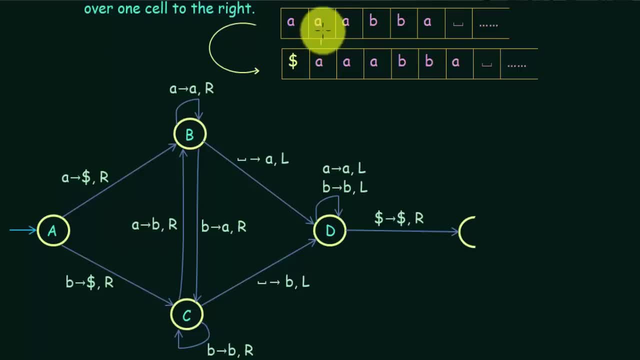 Like, for example: here we are seeing an A, So you replace this A with A itself, So here it is an A, And then you move one step to the right, So we are over here, And you keep on doing this as long as you are seeing As. 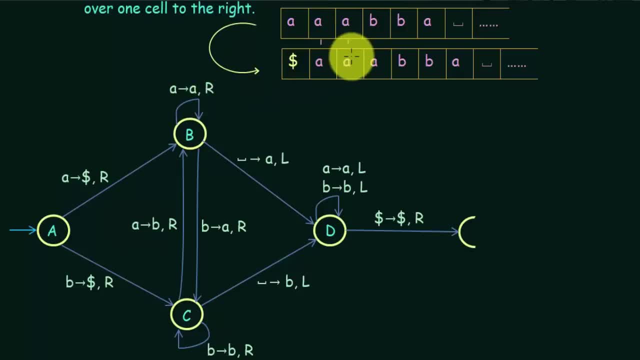 So here also, I am seeing an A, So I replace this A with an A itself and I keep moving to the right. And now over here, what happens is that we are seeing a B. So if you see a B, what happens is that. 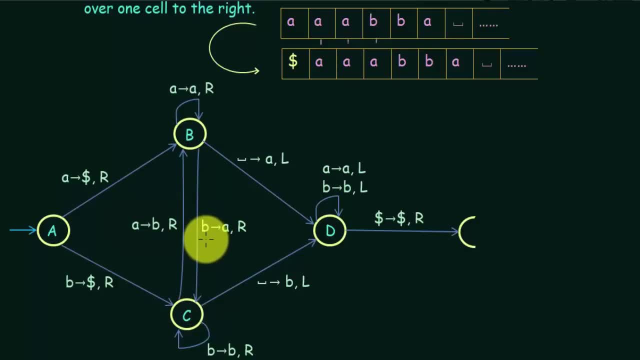 it will go to state C and it says that if you see a B, replace that B with A and move one step to the right. So, even this B, I replace it with an A and then I will move one step to the right. 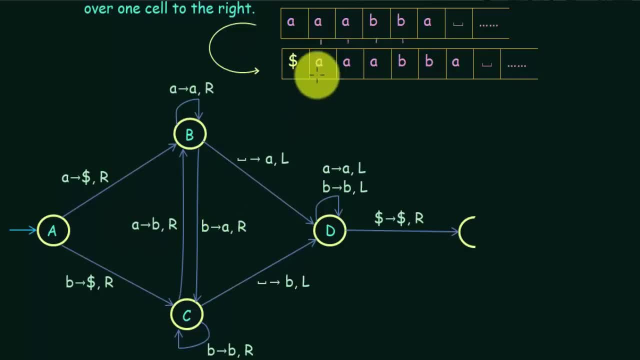 Now why we are doing this is because remember that we are shifting the elements one step to the right. So even if you see a B here, you know that in the original tape that we had the previous element or the element over here it is an A. 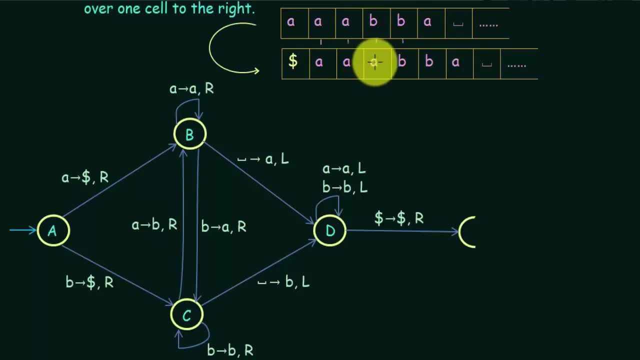 So that is why this B is replaced by A and we move one step to the right. Alright, And in this C, what happens is that if you see B, then replace B with B itself and move one step to the right and keep doing this, for. 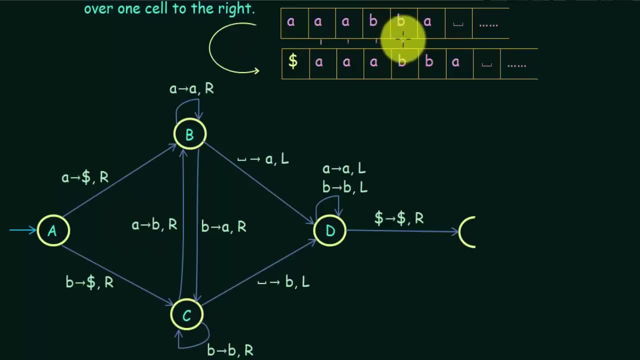 all the Bs that you see. So we are over here and here we are having a B. So replace that B with B itself. So here it is a B and move one step to the right. So I am here right now. 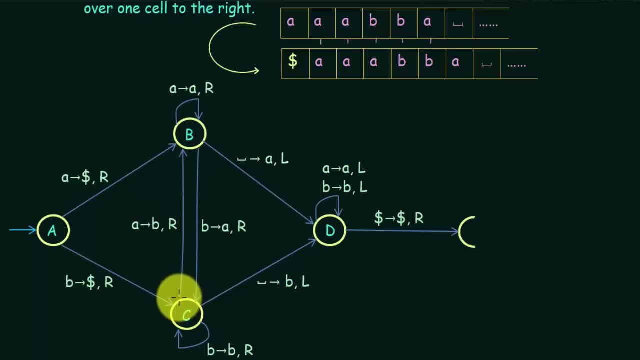 Here we are getting an A. So if you get an A in state C, what happens? Replace that A with B and move one step to the right and go to state B. So here I am having an A, So I replace this A with B. 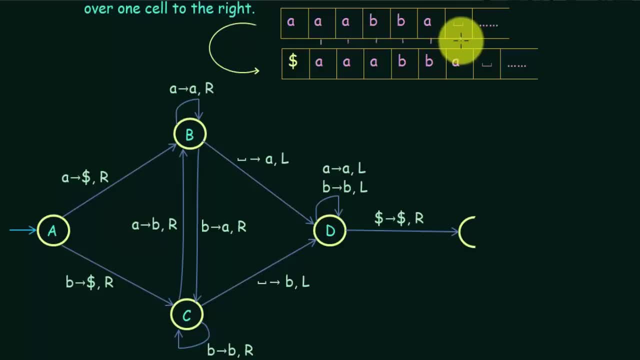 and then I move one step to the right. Now why we are doing this. This is also the same, like the previous condition that I explained, Even though you are seeing an A over here, since you are shifting this whole thing one step to the right, even if you see. 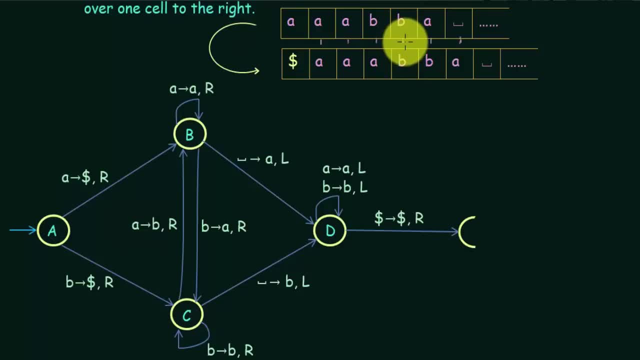 an A here. so what you should write here is the previous thing that you had over here. So you had a B, so you wrote this B and you move one step to the right Now. here you see that we are in state B right now and 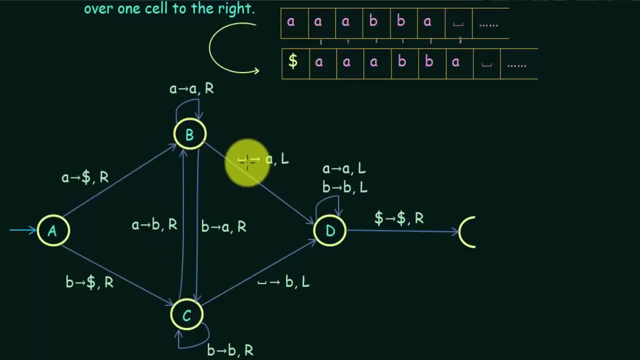 what we are getting is a blank symbol. So in state B, if you get a blank symbol, what happens? Replace that blank symbol with an A and move one step to the left. So I replace this blank symbol with an A, So this blank symbol is replaced with. 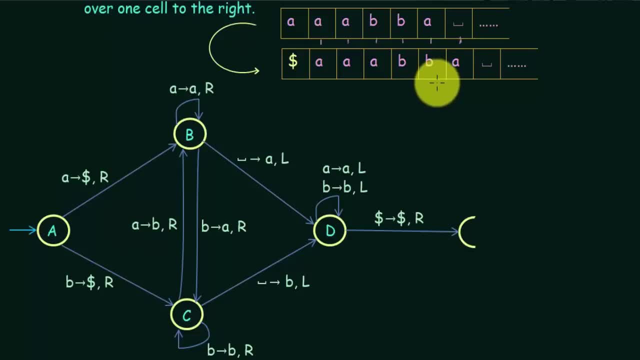 an A and I move one step to the left. So from here I will move over here, Alright. And then we come to state D, and in state D it says: whether you encounter A or B, replace the A with A itself and replace the B with B itself. 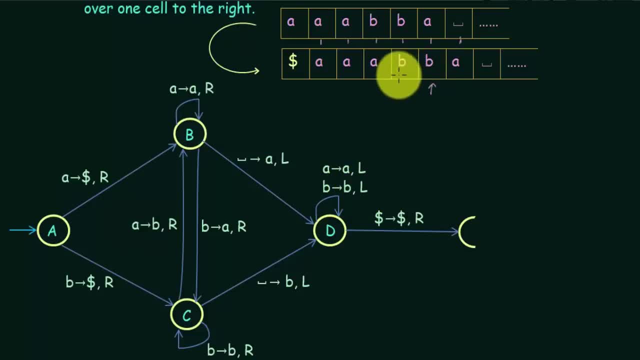 and keep moving to the left. So here, whether you see A or B, it doesn't matter. Keep replacing A's with A itself and B's with B itself. It means that you are not overwriting anything, So you just keep moving to the left. 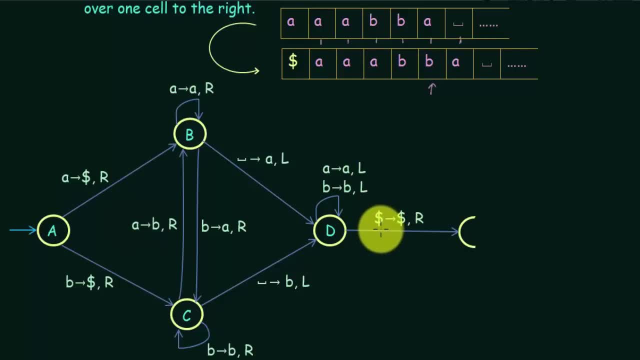 You keep moving to the left until you encounter a dollar symbol. So I keep moving to the left like this and I encounter the dollar symbol over here. So when I encounter dollar symbol over here, what happens? Replace the dollar with dollar itself and move one step to the right. 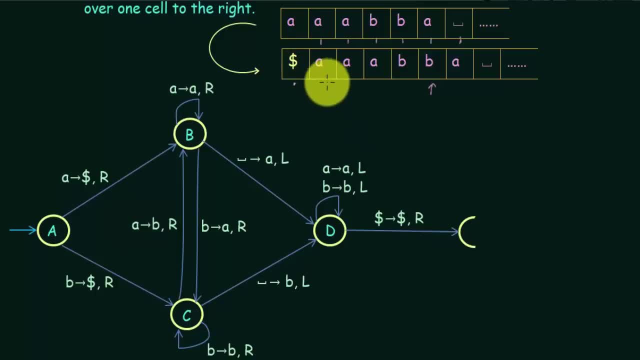 So I am writing dollar here again and I move one step to the right and my tape head is over here right now, and now I am ready for the rest of the calculation, or rest of the operation for which this Turing machine was actually designed. So we see that.